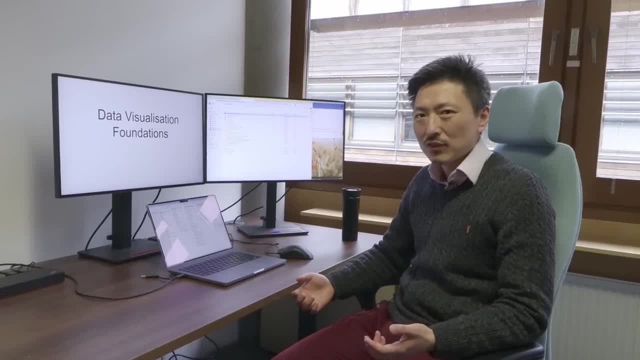 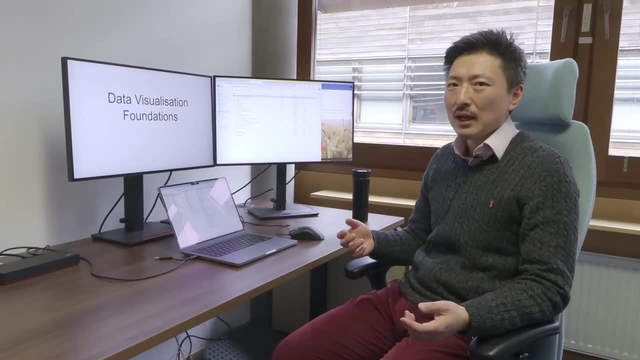 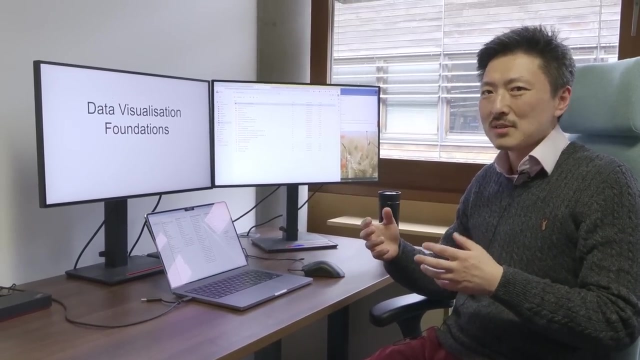 Today we will talk a bit more about the kind of foundations of visualization, in terms of kind of a more simplistic or theoretical way of thinking of visualization and how to use that to design your next realization. So this is not to teach you how to use spreadsheets to create a bar chart, but 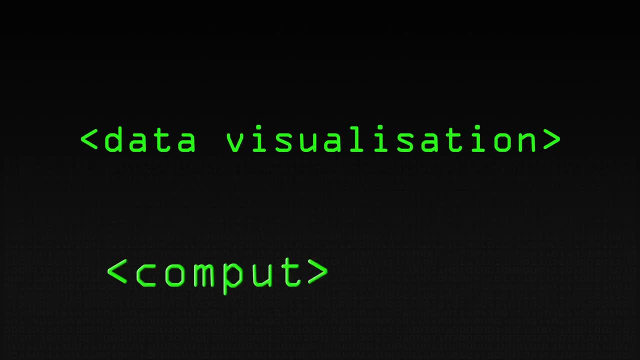 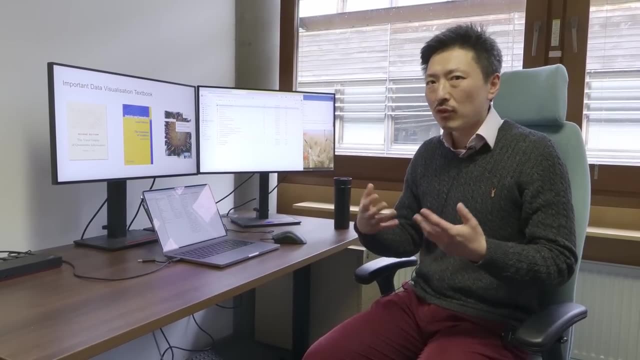 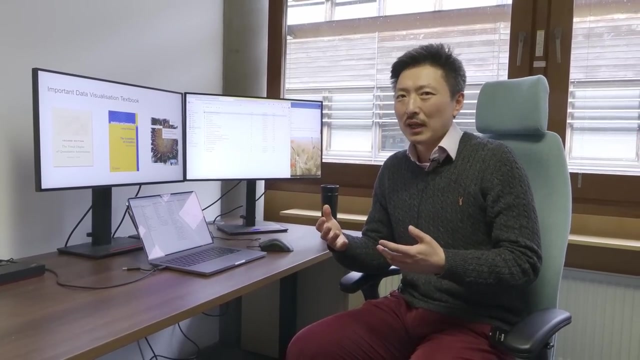 say what makes a good bar chart? The point I want to make here is there's no kind of universally accepted framework or theory about what is a good validation, So to some extent it's almost like art. There's still lots of like, say, personal interpretation depends on particular data or 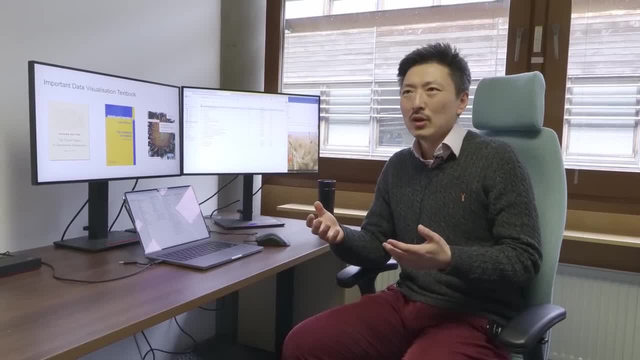 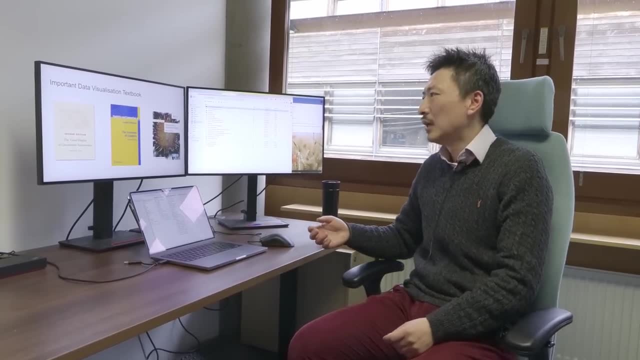 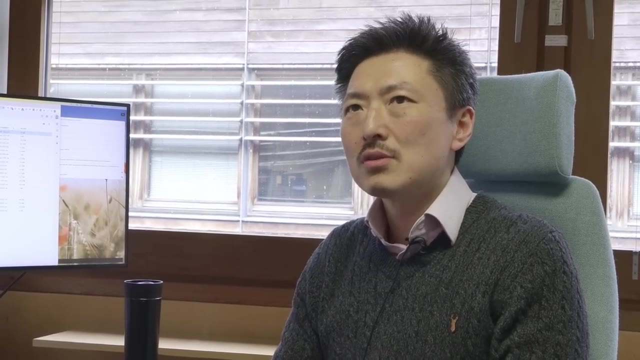 user cases. Just as I assume there's no universal way of writing a good novel, people would have their own implementations, even there being centuries people trying to do that. How is this computer science and not design, then? Very good question. So actually data validation. 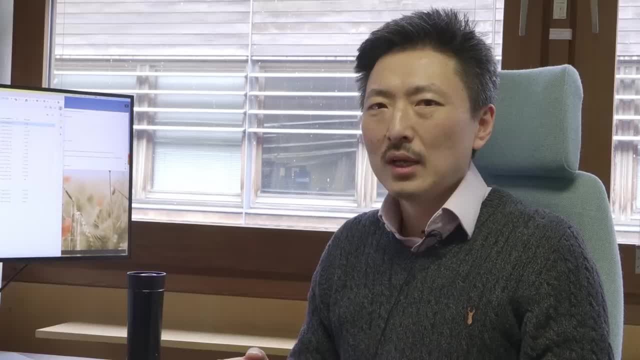 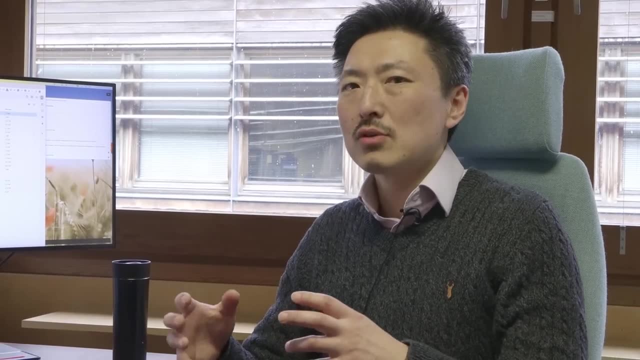 just because its nature is kind of across a few different fields. So obviously even within the computer science it's related to computer graphics, which is more on the visual side, but also the human computer interaction in terms of how people use it, And in my work actually, I 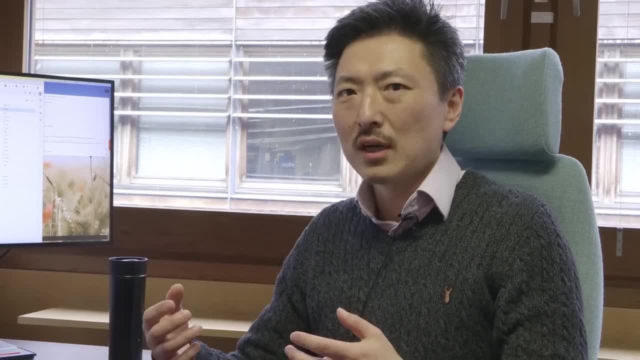 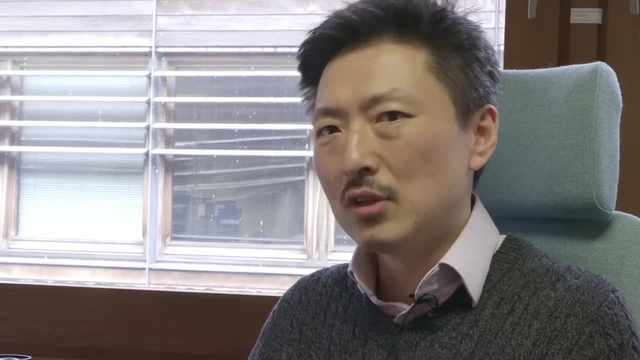 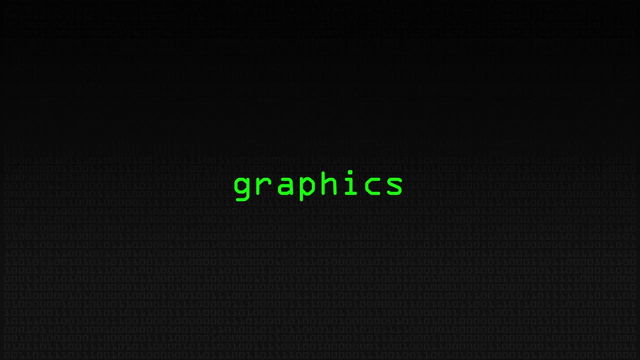 see, quite a few colleagues from the psychology or even neuroscience department or the understanding, the more fundamental thing, for example in the human brain part, how would they see reacted to different visuals. So it's kind of very cross-discipline thing. So today I really just only want to cover graphics, which are the things, visual things you see on the screen and 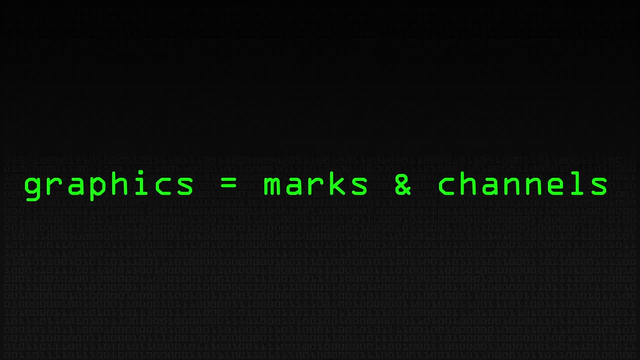 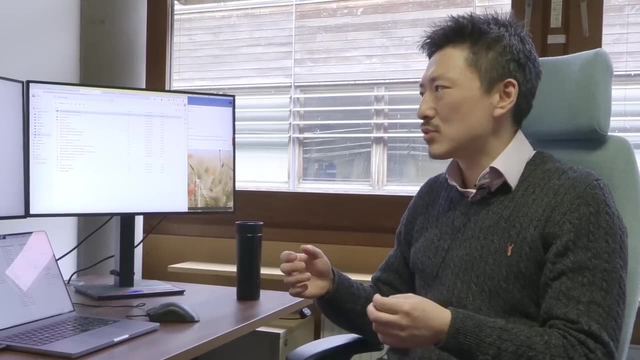 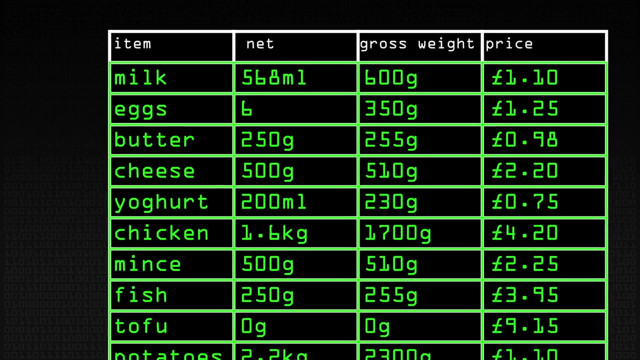 it's composed of two parts, and one is called the marks and the other one called channels. These might be called different names in different contexts or discussions, and the concept here is probably the more important part, And so first and marks is what I would call data items. So let's 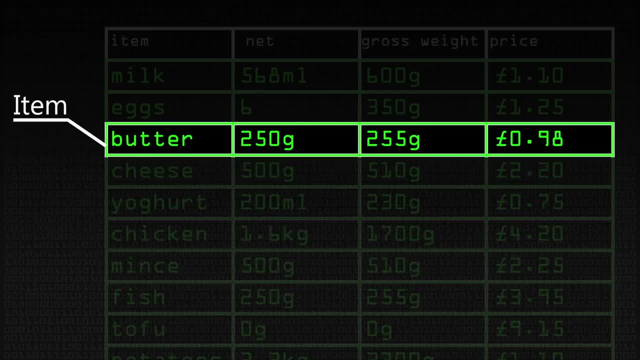 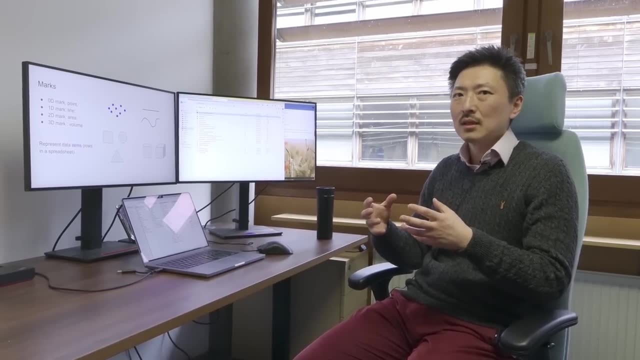 assume you have a spreadsheet which lists all the products in the supermarket or shop. So each row is a product which is an item. So these can be represented visually as a mark And so you can imagine you can potentially use a point to represent one product. depends on what the 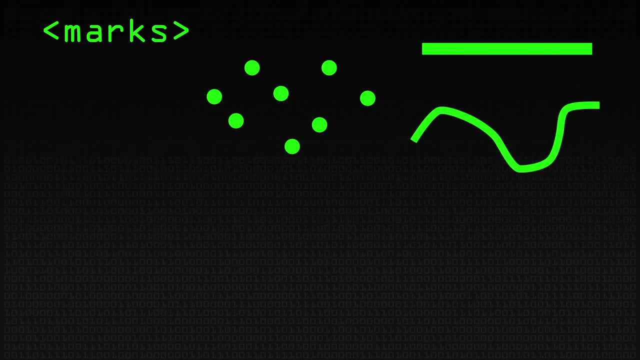 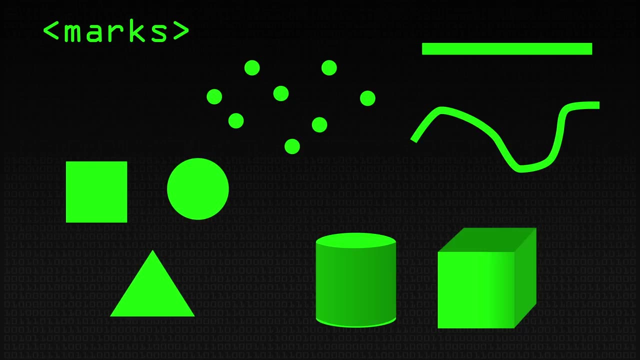 visualization is maybe a line in a bar, chart, a bar, or you can have more fenced representation for each product and, as say, the shape, or even 3D shape. You can have different dimensionality without the mark, but this really represents one data item or one entity, So that's marks. 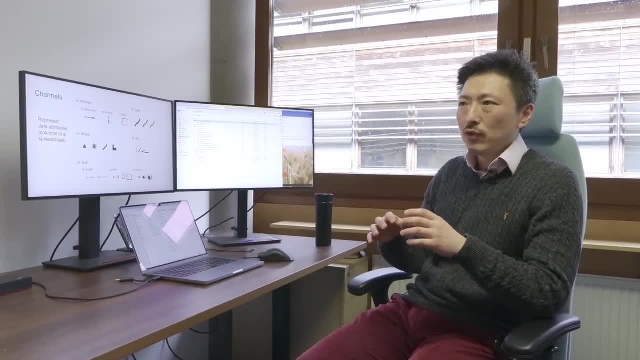 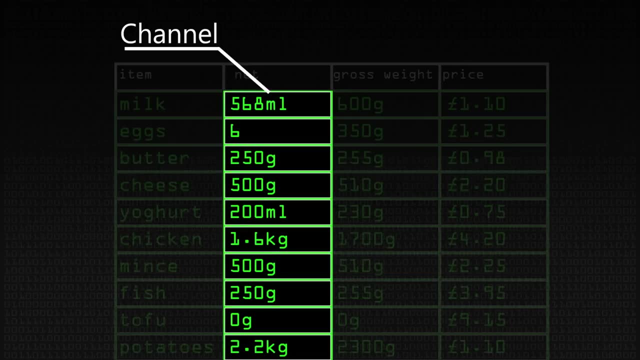 And then there's the other one, called the channels, which is the visual representation of the attributes of the item. You could say you can think about a product. it has, say, the name, the weight, and it will be associated with information like the sales or profits. 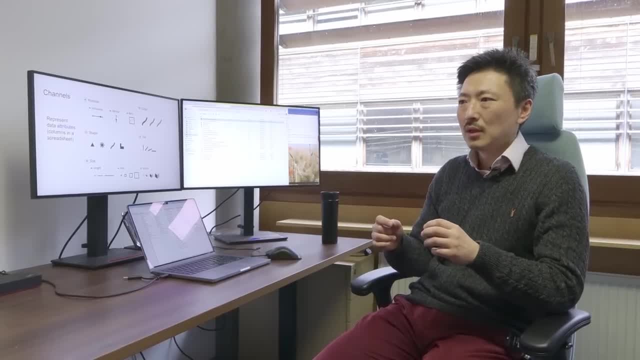 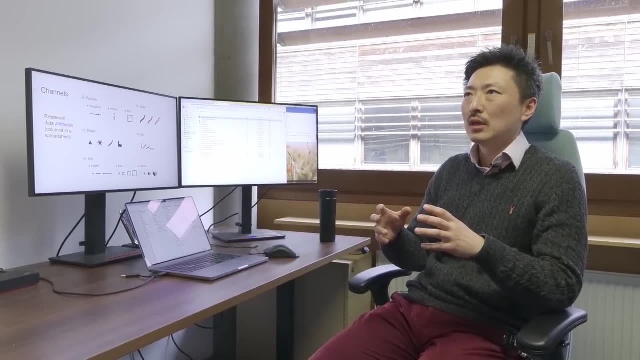 these kind of- I call- attributes of the items, And usually it will be the columns in your spreadsheet, and these are the things you probably want to also include in your visualization as well. So you want to show the product and then other information associated with the product, like the names. 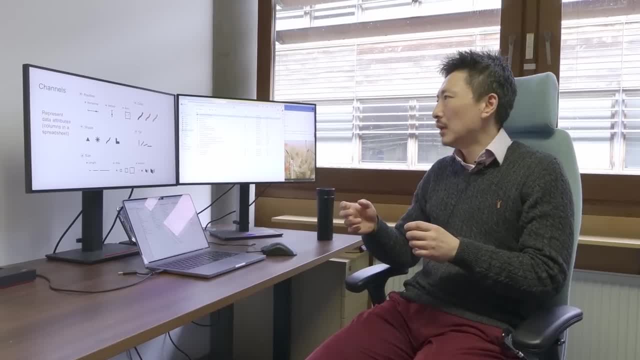 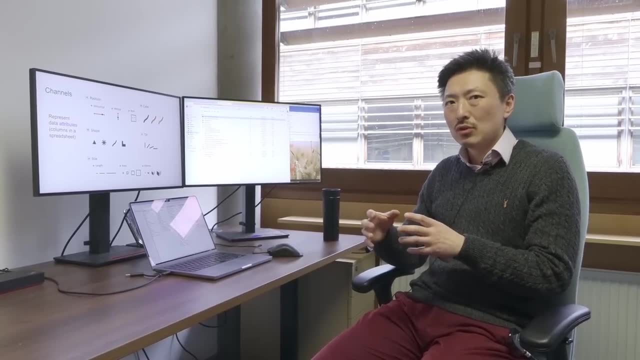 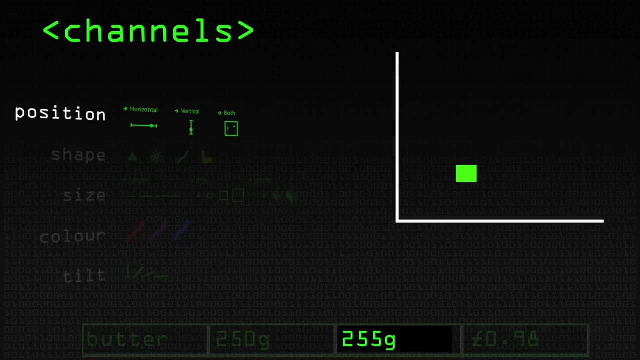 the price, the profit and so on and so forth. and so a large part of the visualization is just say, mapping the attributes to the visual. so I say I want to show the price. then I can choose to use, say, the color or maybe the size to 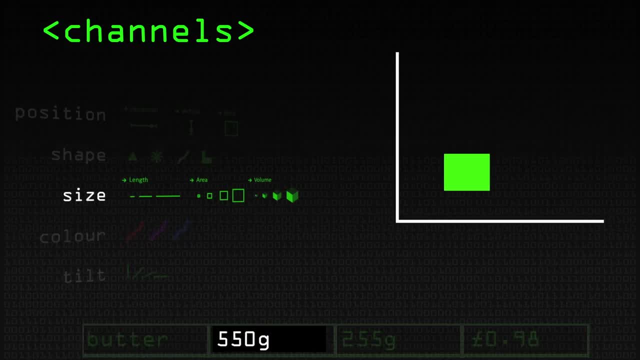 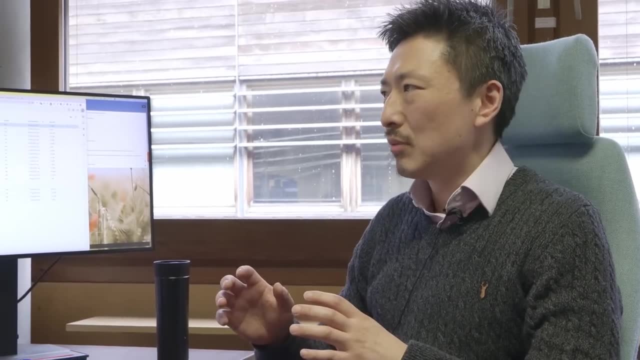 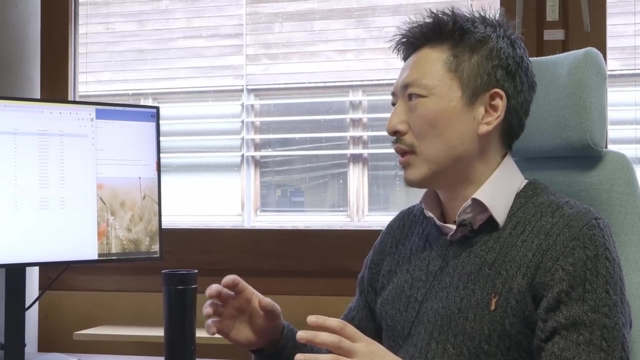 show the color, then there's a choice there, and often there are more than one attributes you want to show and then you have a choice between which one to use which channel. just taking a very simple example to explain this. and so if this is like a scatter plot and we have some showing the some kind of product, 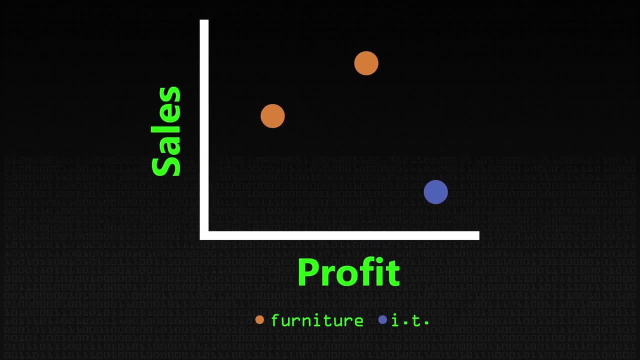 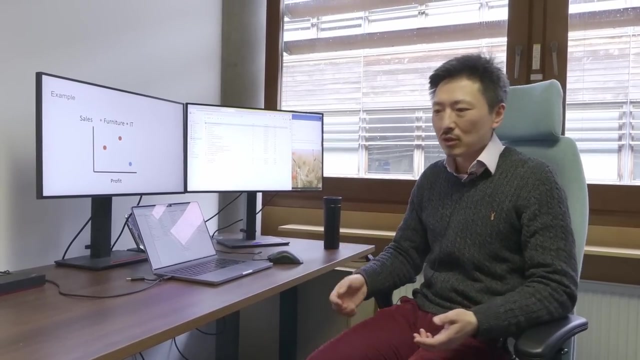 information and we showing the profits of each product, the sales of product and then the type of product. so it's showing three attributes in the data. we are using a 2d graph because and the color itself is not a spatial dimension, but also that's usually actually a good thing. 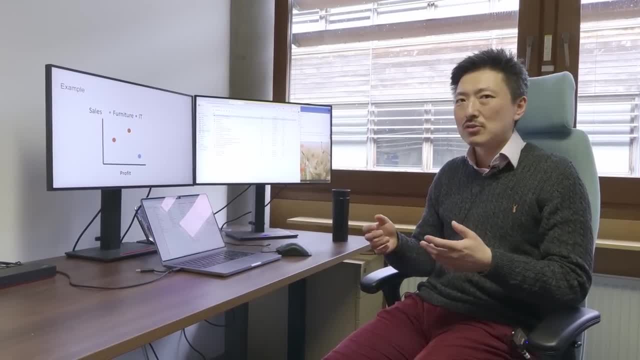 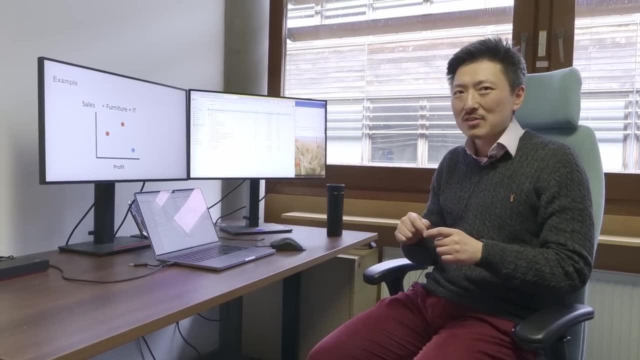 but also that's usually actually a good thing, because if you're not limited to spatial dimension, that means you can be on 3d, so you can go say five, six, seven, ten and so on, so forth. okay, and then back to the marks and channels. what are the marks here? okay, the marks are the the. 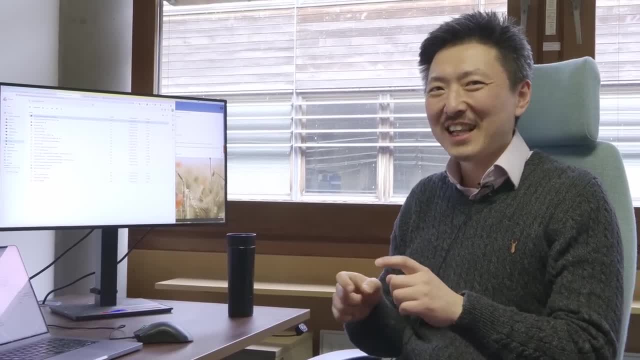 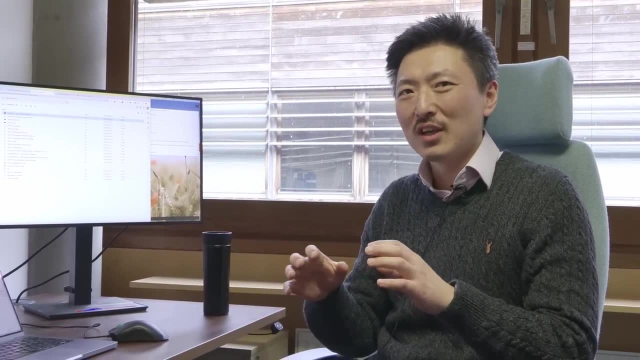 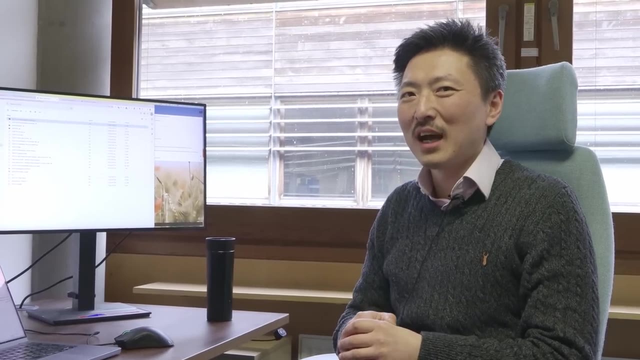 type, the colors, basically. is that right? I think that's the channel. so marks is the one, exactly exactly so. the marks represents each items in this world will be the, each product, which will be the dot, and then the channels. we already said color, color and also the place on the graph. yeah, exactly so. I mean more formally, we call 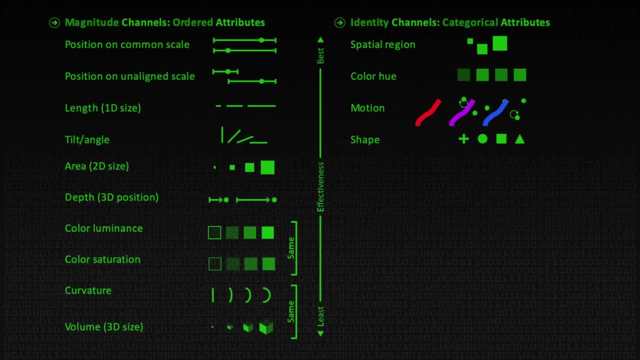 these positions, basically x, y, coordinates or the positions. so this is looks a little bit busy, but really show you. it just says: okay, when I have some attributes that I want to show, for example the price, what will be the best channel to show? do I use position color or 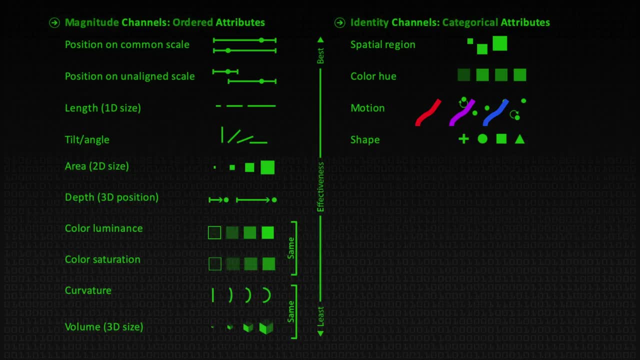 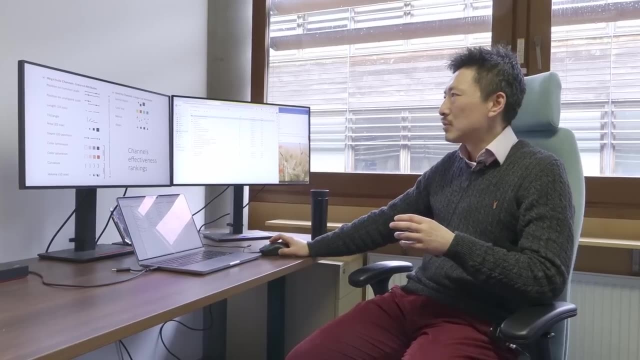 maybe 3D or maybe tilt the levels. yeah, so I'm not going to go through the exact list, but generally what people did is did lots of experiment. for example, they want to find out whether you use position is better or using color is better. there's lots of small experiments. 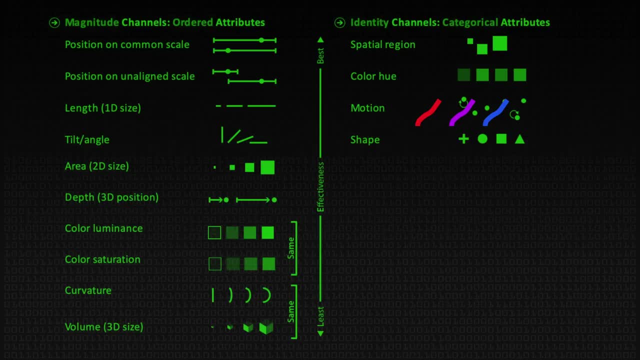 the pairwise comparison they kind of eventually become this list and it's not second absolute order. for example, these two say: either using the luminance or the gray scale or use the saturation level of the color they have come. similar level of effectiveness. so the further on the top is, the more. 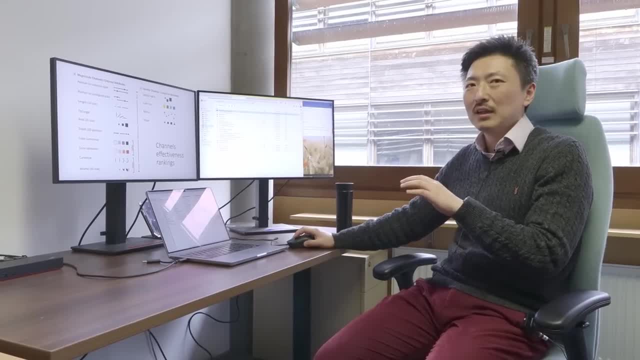 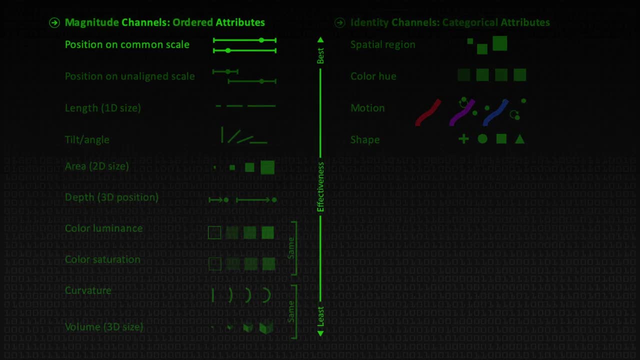 effective ones in general, at the bottom are the less effective ones in that particular order. so very quickly say: the position x, y is actually very effective and then say: for example, 3D shapes is usually not very good, so at least in academics is a big part of the. 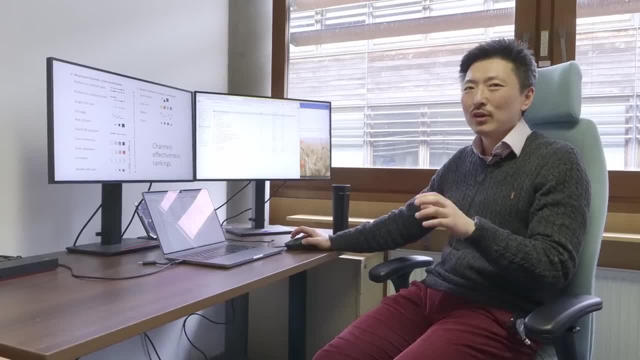 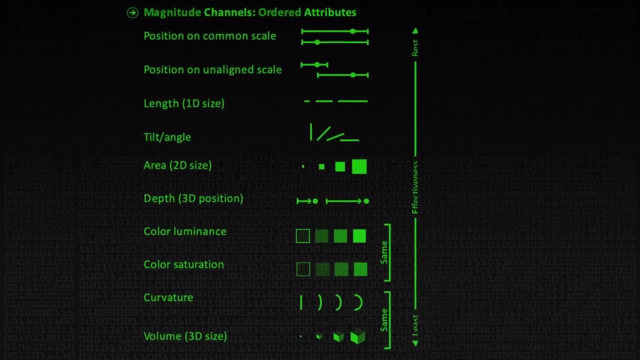 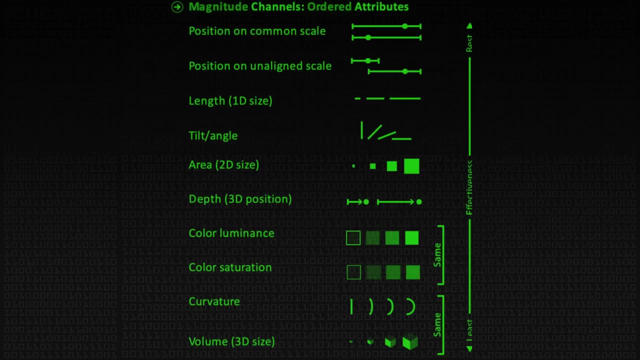 visualization research community think you probably should try to avoid 3D if you can, just because it's not very good at representing. and also we have these two parts, so the left part is to represent numbers basically. so these are type of data you can say represent. you show a number, say price, profit. 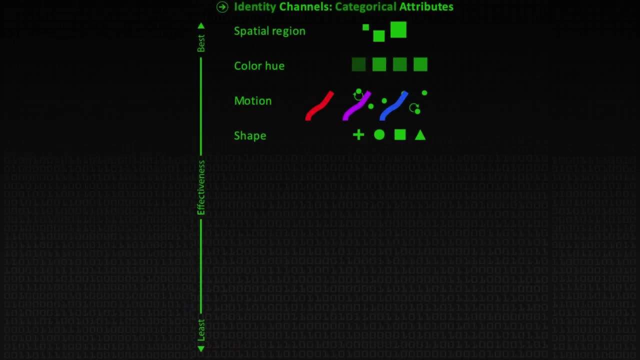 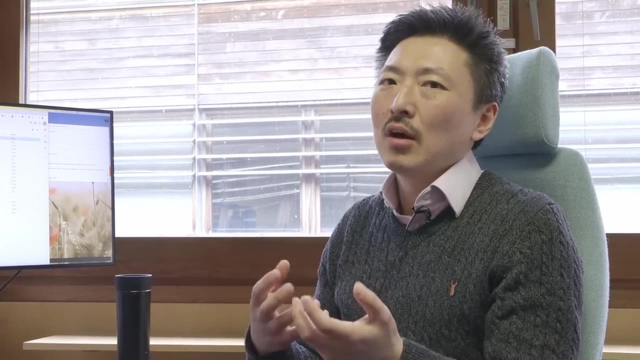 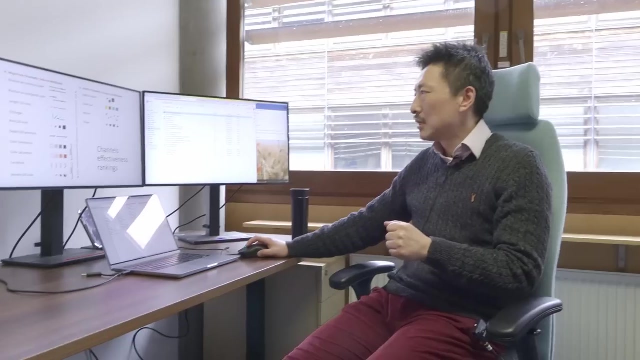 and on the right hand side is the more categorical type of values. for example, different type of products, say they have, they have distinction, but they can't really do anything. any operations. they're not usually a number and again, so there's a limited number of channels usually can be used. 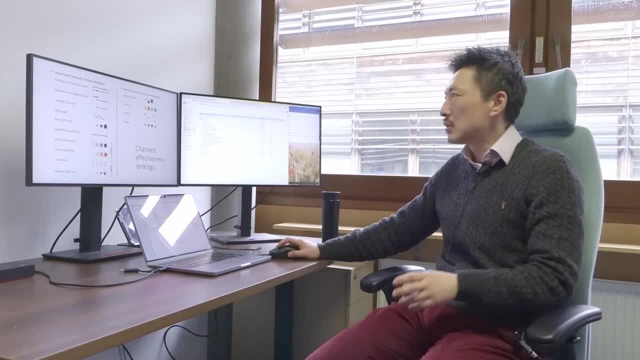 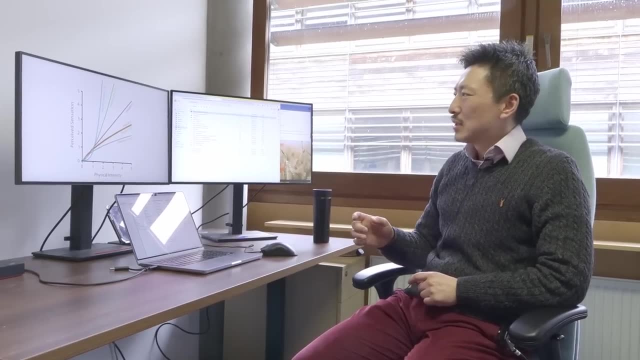 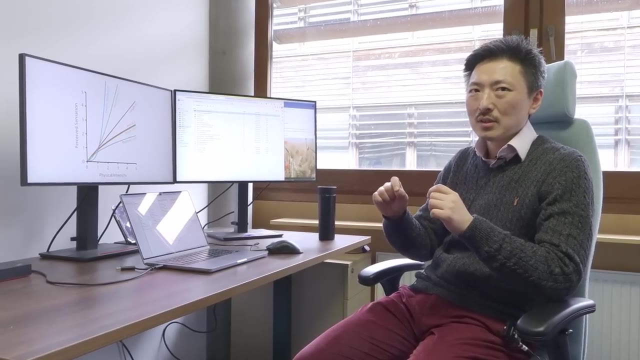 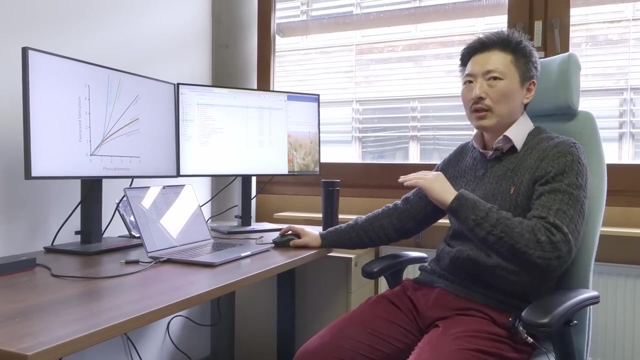 for different type depends on type of attributes. the effectiveness is also a little bit different. okay, yeah, and so this is. people do experiment, try to understand how accurate a channel is, so each line you have is one channel and then, so this one would be the actual value, the x-axis. 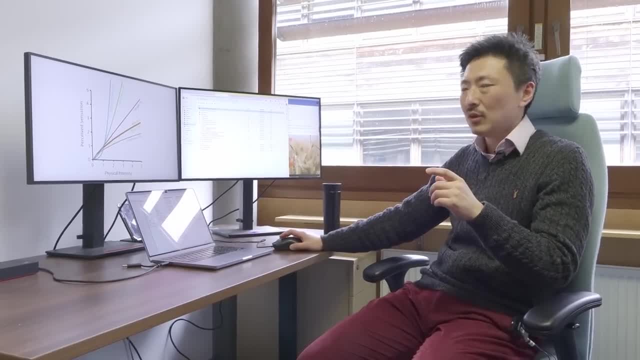 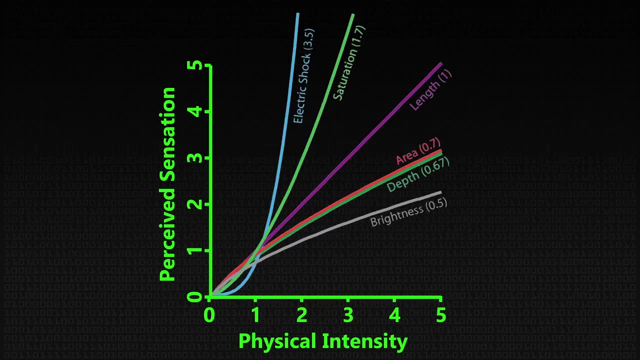 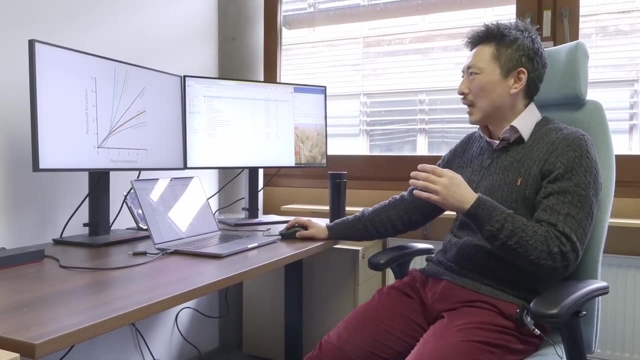 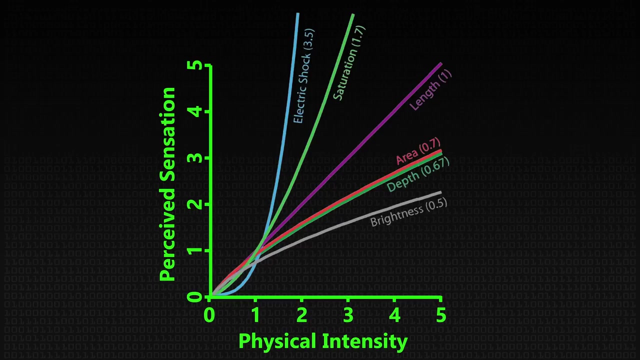 and the y-axis will be the perceived value, and so you can see the purple line here is lens, essentially the position. so the actual value is very similar to the user perceived values, so which is a good thing. so anything under this, for example brightness, that means people underestimate. so if, for example, 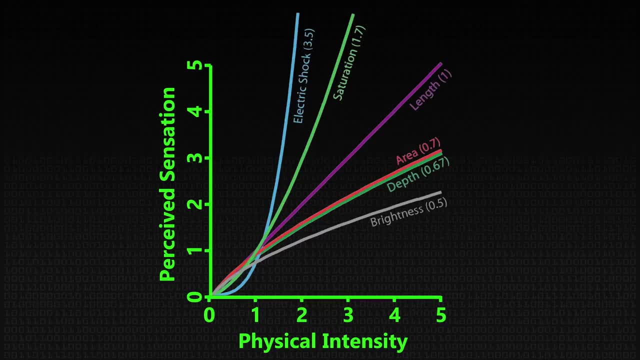 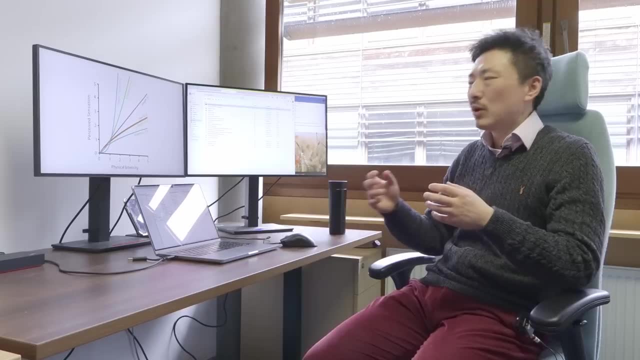 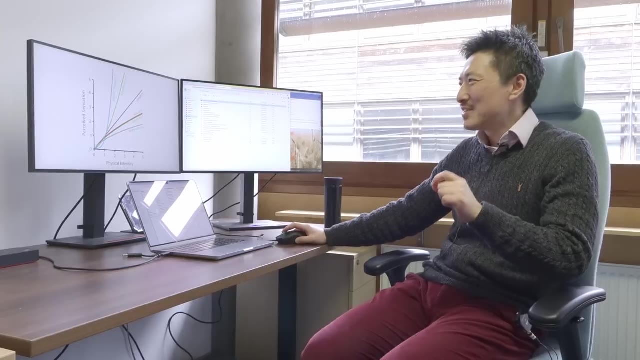 if you make twice as bright, and then people maybe only think it only increased by 50 percent, whereas on this side, above this purple line, are the ones which people overestimate, and so what they include here is electric shock. so if you're increasing voltage by just a tiny bit, the 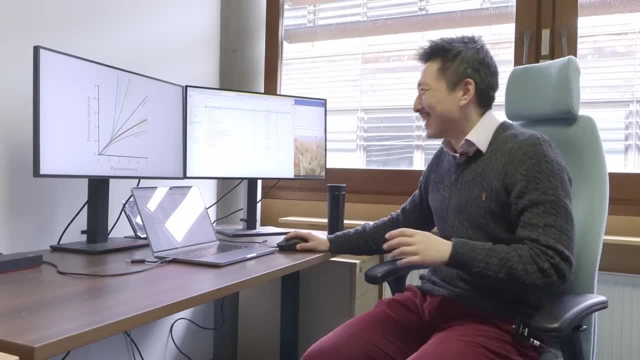 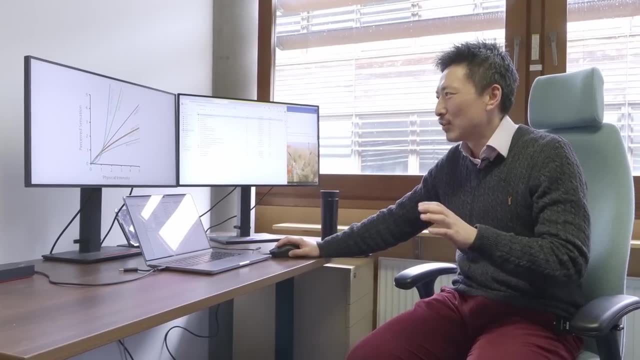 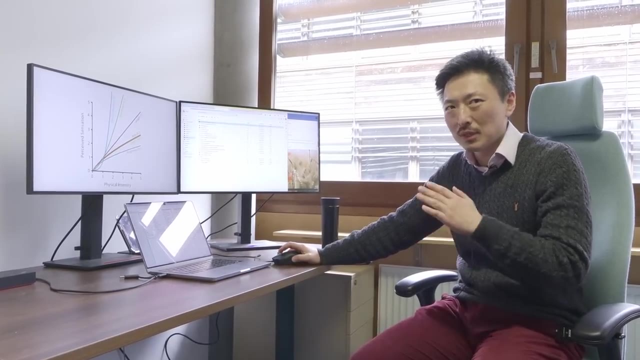 people feeling is way, way more painful. yeah, you have a number there which is 3.5 times more painful, but yeah, but I think the more important thing is just the kind of general thing you over and then estimate, and also the important thing is you try to be in the middle as much as possible. 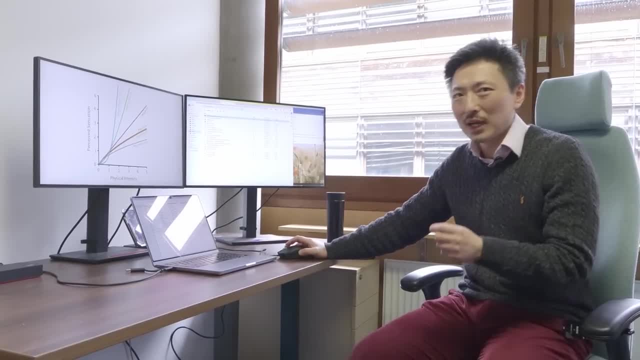 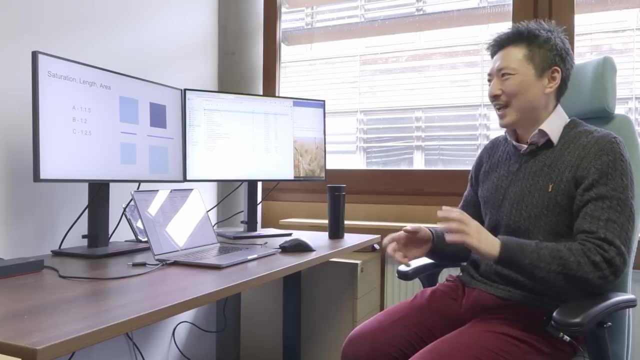 that which give you an accurate estimate. otherwise you have to kind of actively compensate for this, which is not what we usually do at human okay, and so this is the last one. so we're going to do one of these little experiments we mentioned earlier on, just to see how accurate 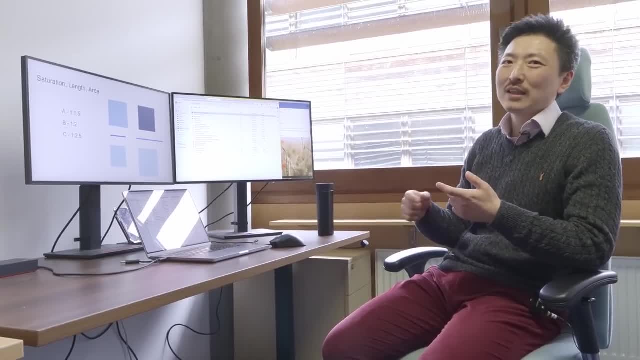 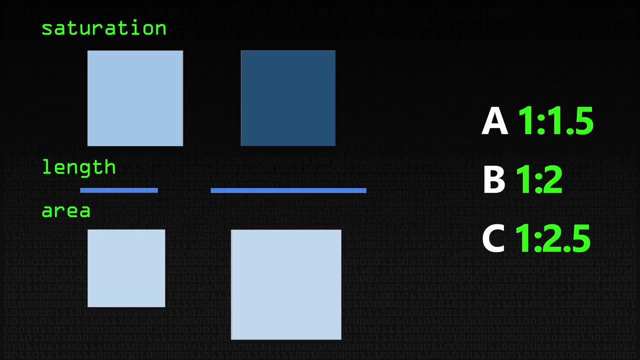 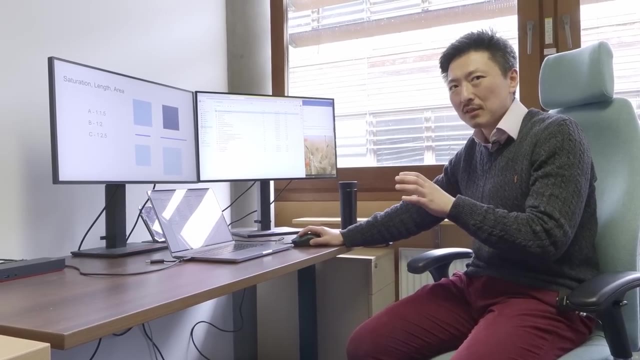 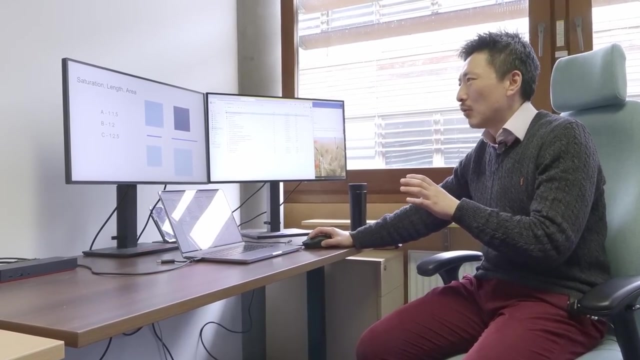 we add human and do we actually tend to over underestimate the visual representations. and so I have three representations here. so we're all representing a number. so the first one: I use color. so I use, say, the darker the color, the bigger the value, and they're going to ask Richard to pick, say, do you think this one on the right is one half times? 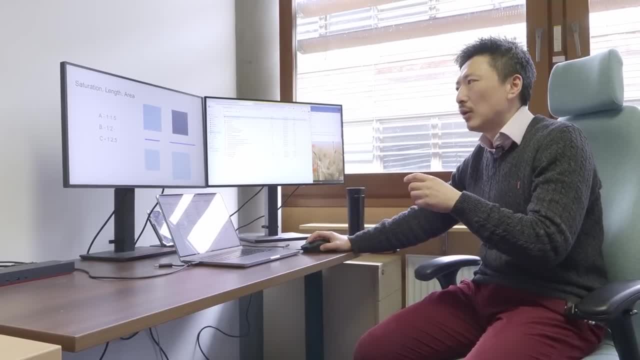 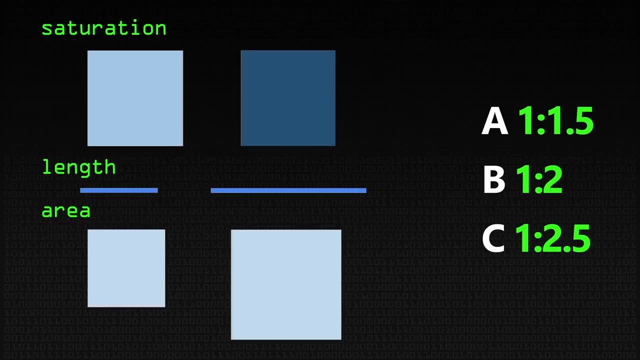 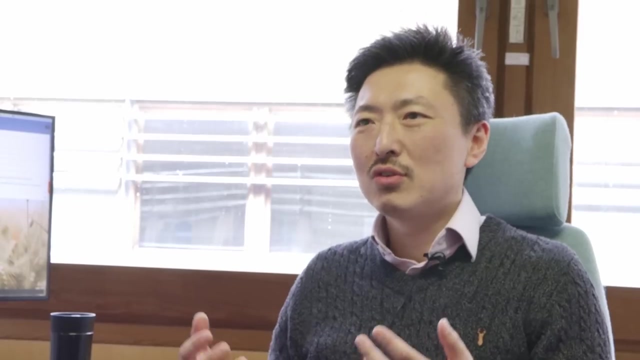 bigger or darker, or or more saturated, or or twice or two and a half times more saturated compared to the color on the left. um, so if you're trying this yourself, I would recommend try not to think too long about it, overthink about it, because when you usually look at a realization, you will not 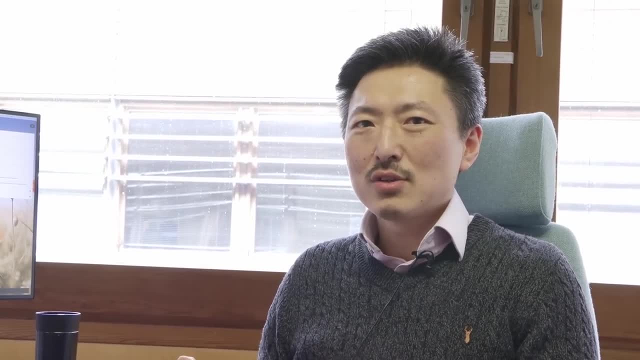 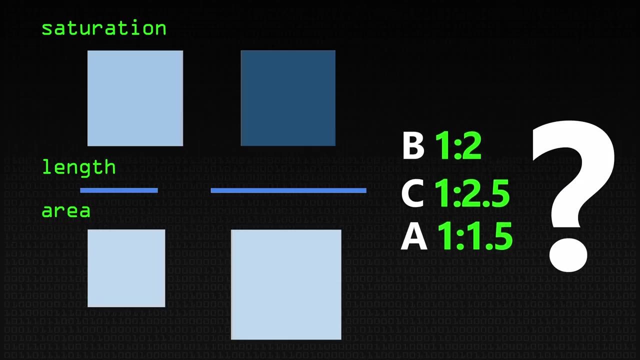 think about is it accurate or not, or question your decisions. just take your kind of instance and gut reaction and go with it and I will show the answers after this. but if you're interested and you can put that in the comments, what do you think it should be? I'm 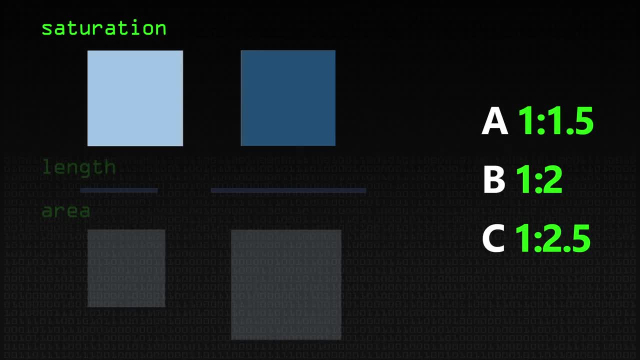 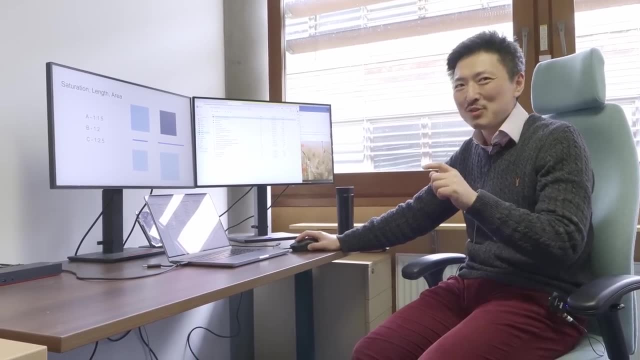 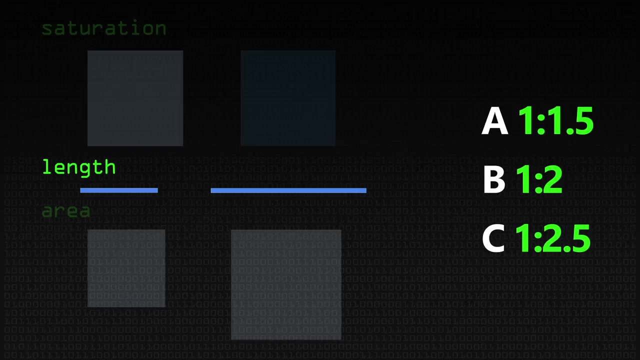 going to say sorry, this is darkness, is it? yeah, so darker means more, larger value. I'd say twice to two, okay, we're going to do over these three and then come back to look at it. yeah, and then this one is using Lens, so, and a half times, two and a half times, okay, and this one is area. the last one: 1.5, 1.5, okay. now. 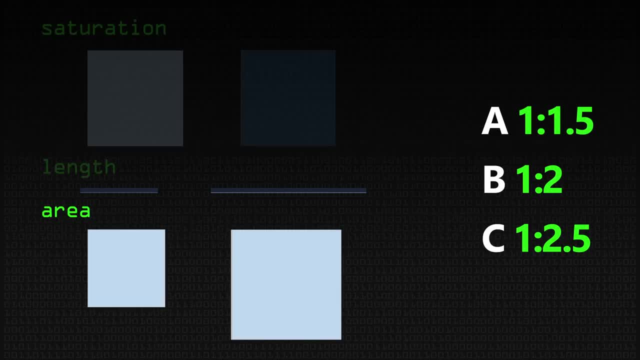 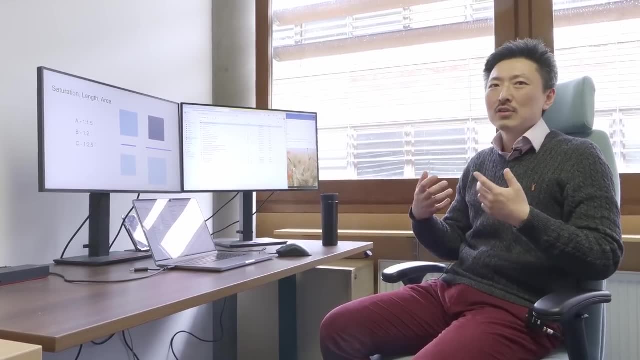 i'm looking at it and i'm changing my mind straight away because, no, no, don't think so. this is the important thing. so the key here is not to think too much and use, um kind of your first intuition for reaction, because- and when you look at the actual data validation, you probably would. 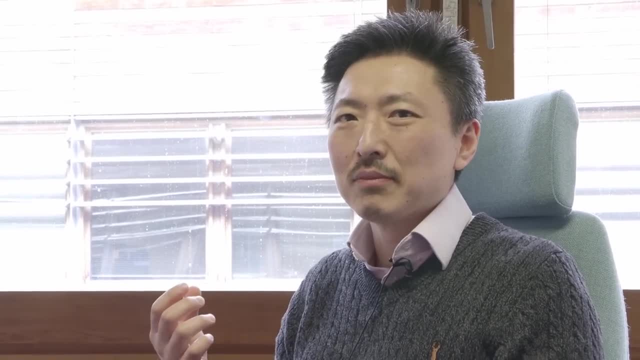 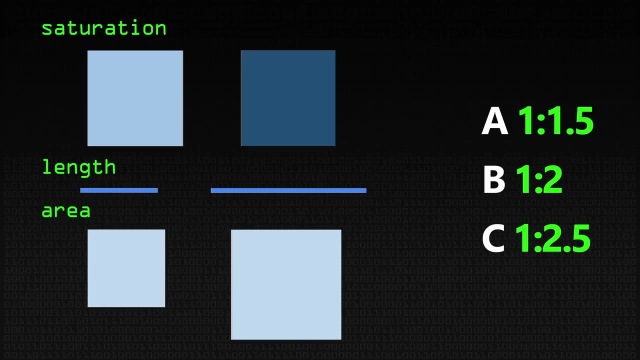 not just think about it really, is it just say you'll have some impression immediately, then that will be answer. most of the time you were not going to kind of carefully think about the question of your choices, so the answer is actually: it's always twice. oh, they're all twice, always twice. 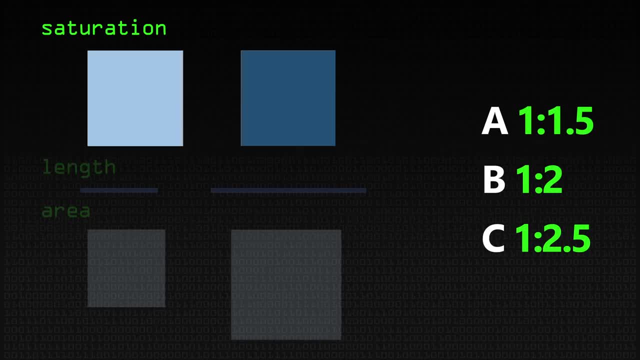 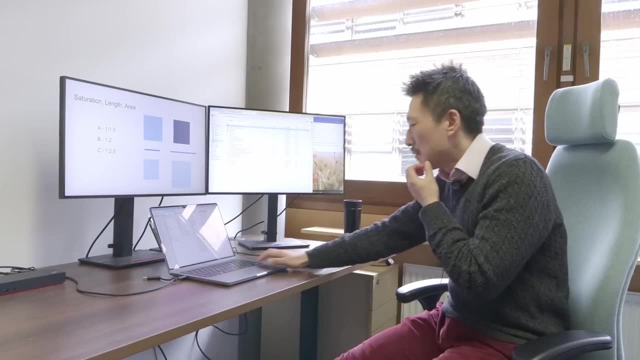 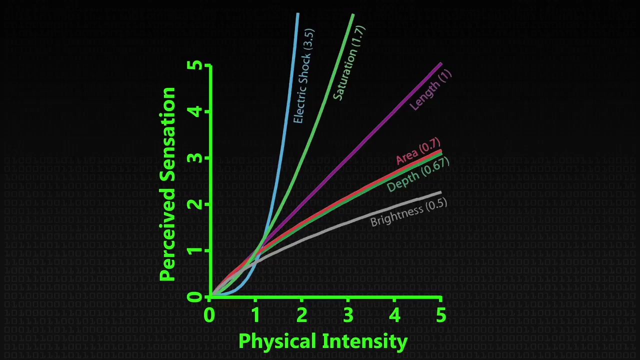 okay, and so i mean quite a few times. people actually overestimate this part as well. so you think maybe it's more than twice darker than this. obviously you can set the rgb values if you look at the here before. so the saturation is about here. so it's people tend to overestimate. 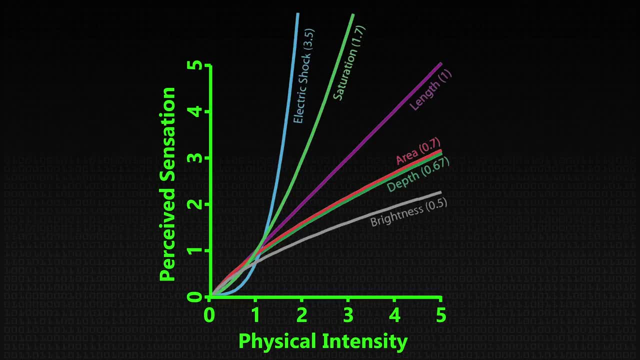 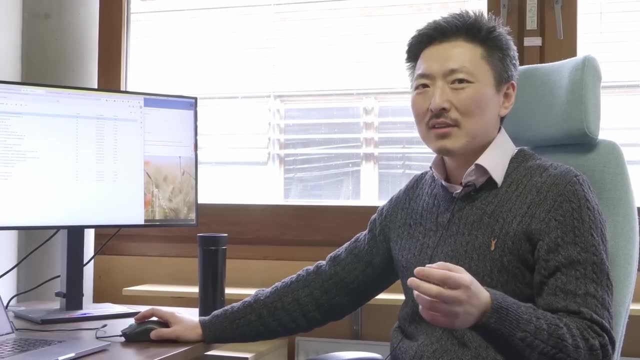 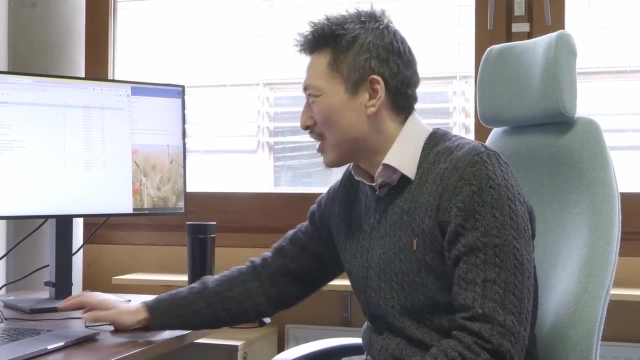 and then area is here, but people tend to underestimate. yeah, so again. so it doesn't work for everyone. I think even I do this in class or I have, like it, sometimes close to hundred students. each person would have slightly different accuracy for these channels, but but in general I think these are kind of much larger scales experiment. 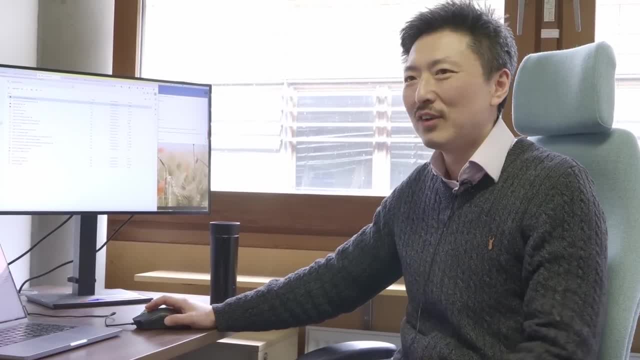 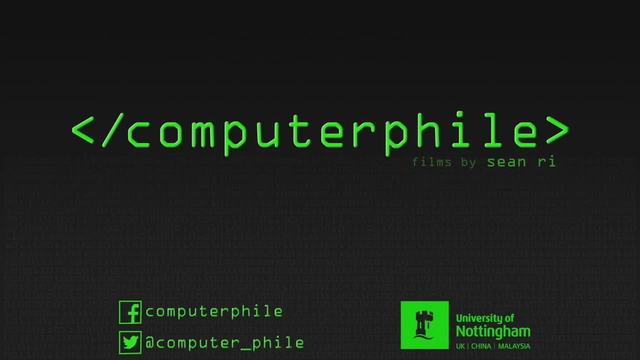 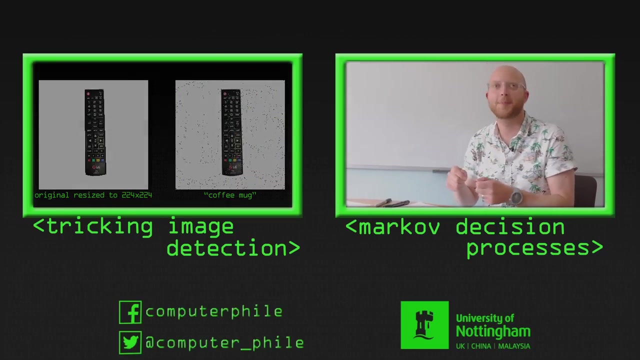 with hundreds or even more people and then has been kind of revalidated afterwards as well. so that's usually accurate. all the changes that is made to the image. it now thinks that that is over 99% like it being a coffee mug. can you see the coffee mug there? if it is, it's the way we solve this is with.